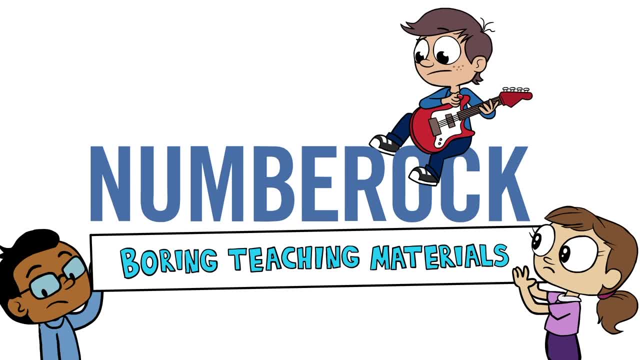 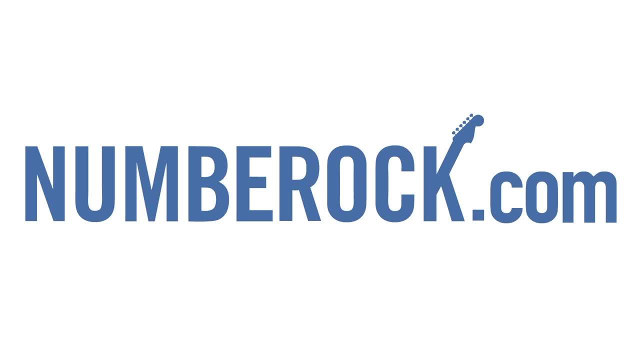 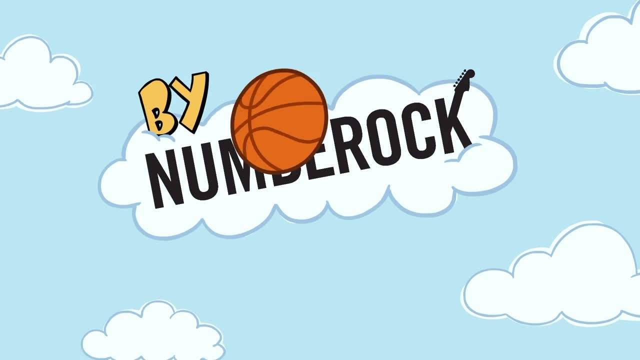 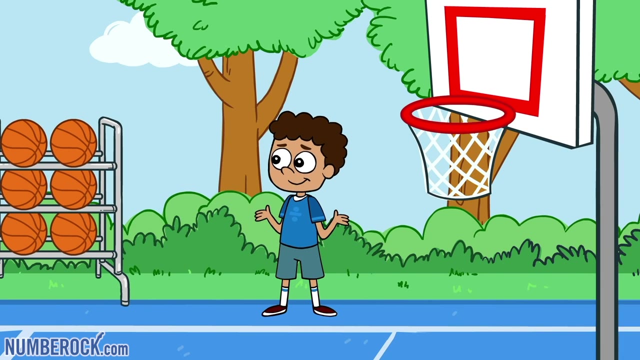 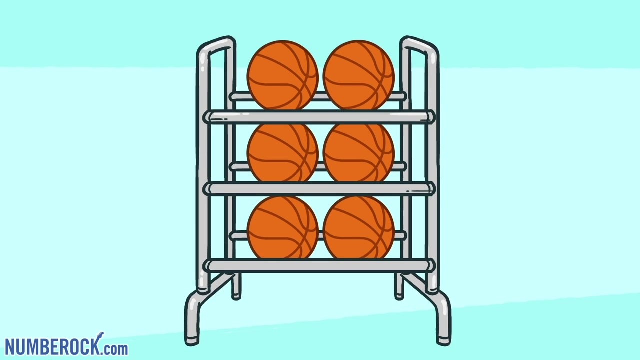 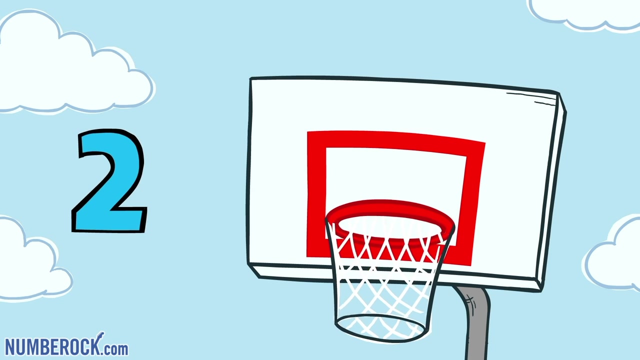 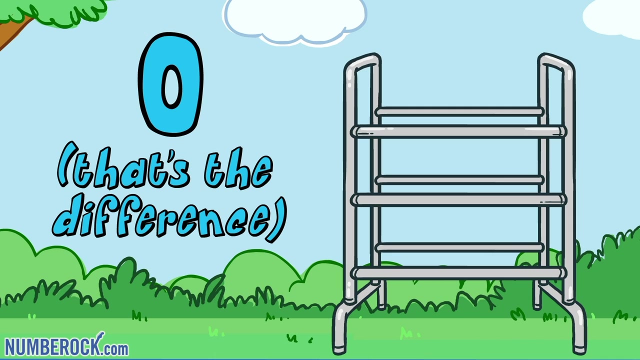 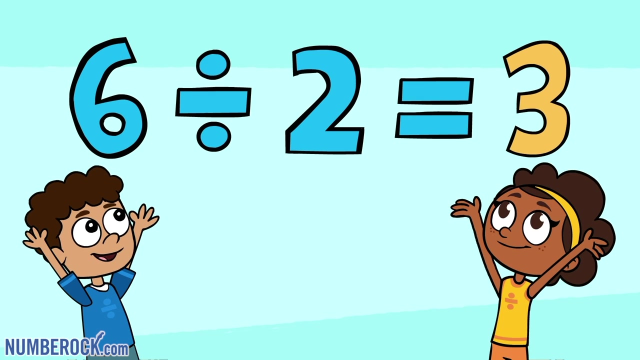 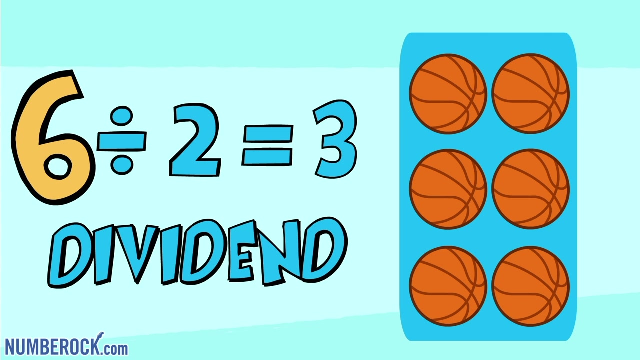 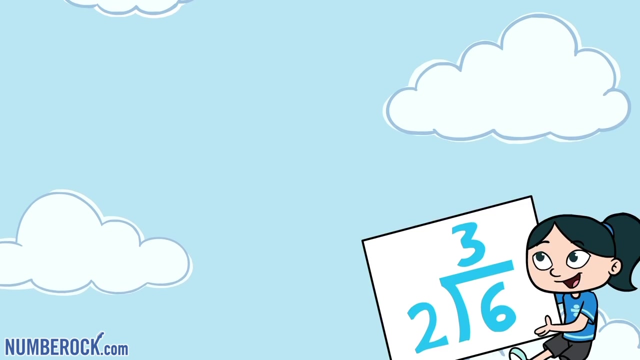 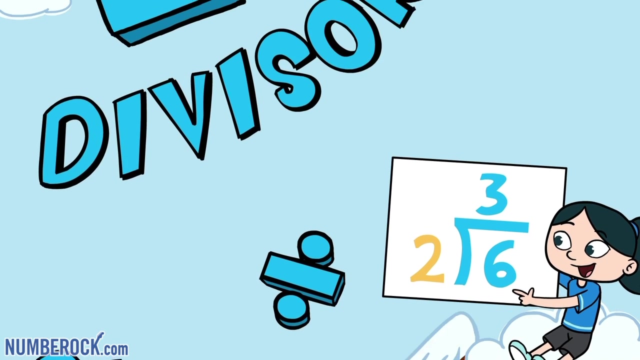 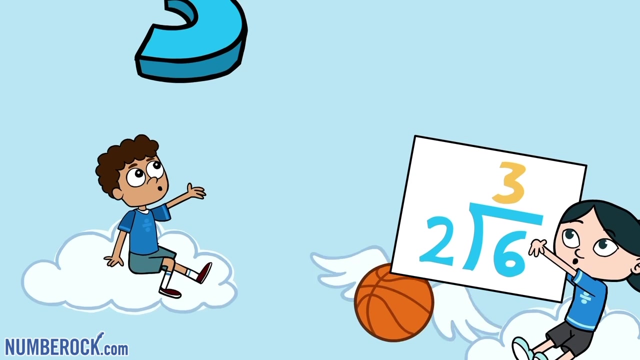 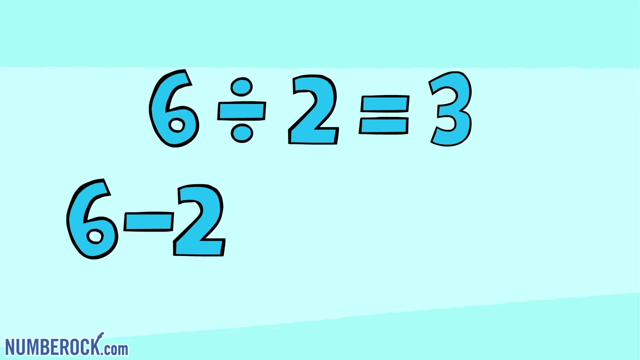 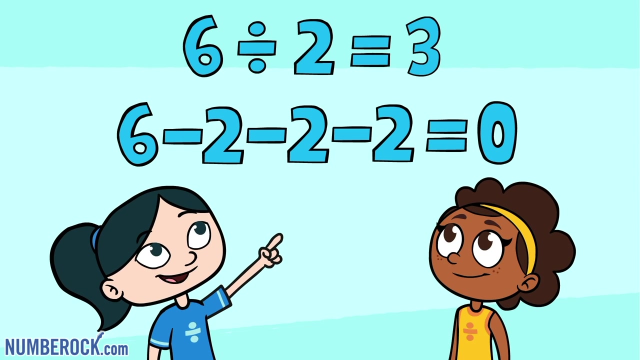 Get on over to Numberockcom for some very not boring teaching materials And add free videos. Numberockcom Subtitles by the Amaraorg community. Subtitles by the Amaraorg community. We can think of six divided by two as repeatedly subtracting groups of two from six until there are none left over. 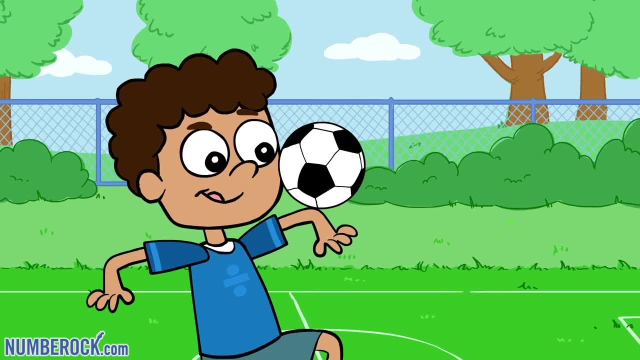 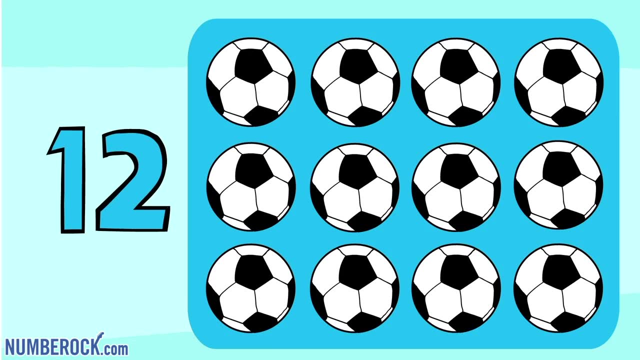 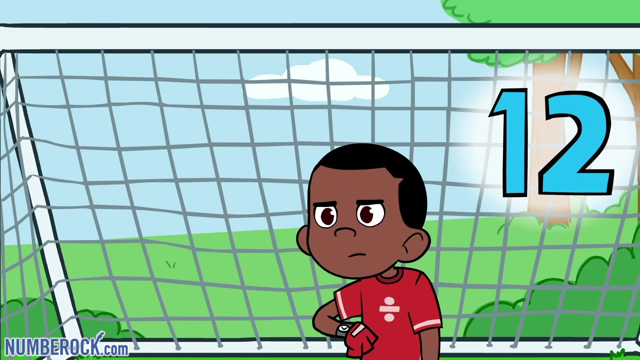 Let's go. I was practicing my aim Before the soccer game. Four groups of three soccer balls, Twelve soccer balls in all. I got the first group of three in the net. Then, again and again and again. It was a perfect set. Now, zero balls are left. That's the difference. 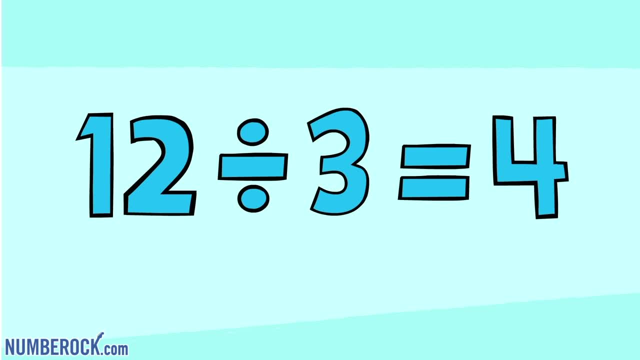 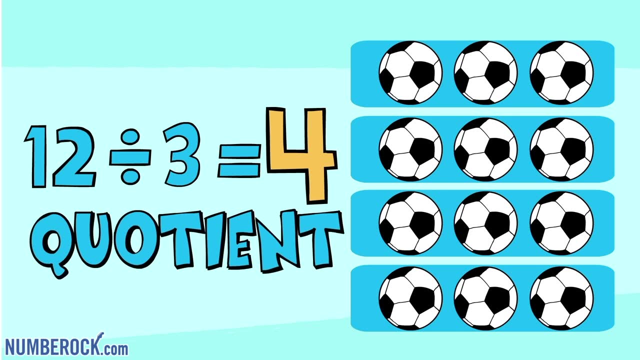 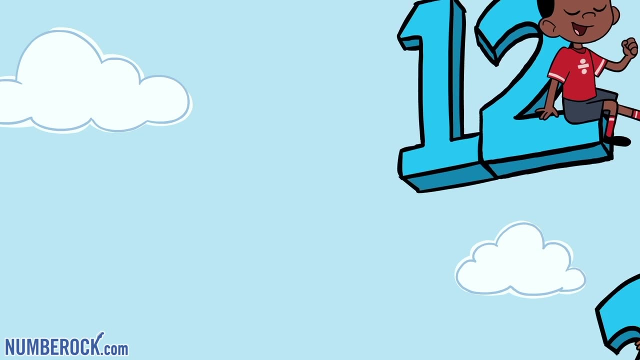 And we can show this as a division sentence. Twelve as how many groups of three soccer balls. We see four equal groups in all. So we call four groups the quotient, Three the divisor and then Twelve the dividend. Yeah, yeah, Ooh, yeah, yeah, yeah. 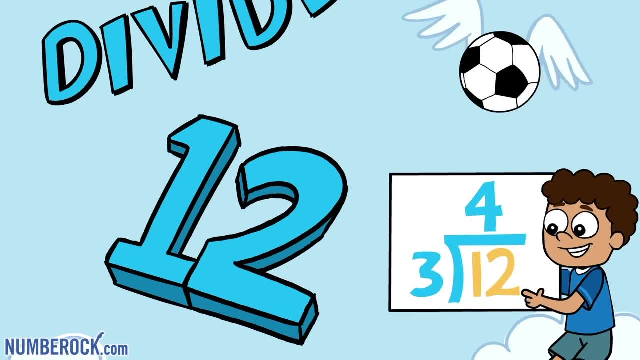 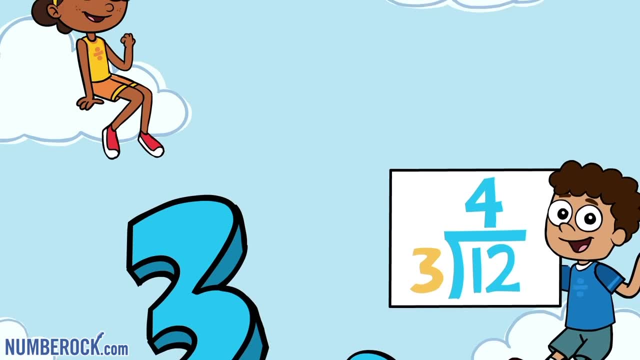 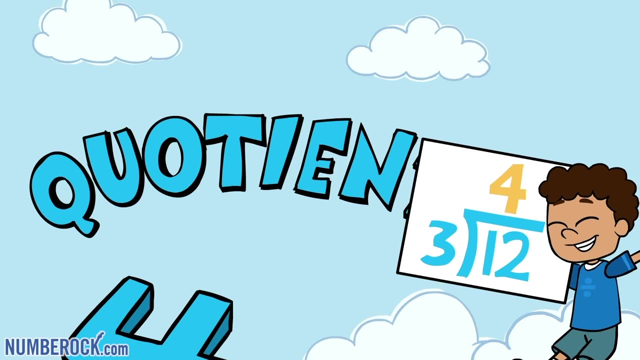 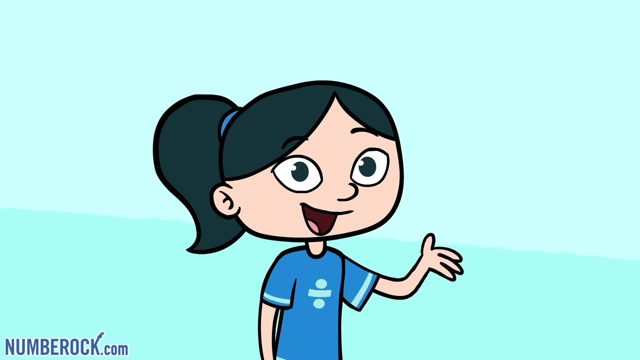 The number divided Is the dividend. The divisor divides So that in the end We find the number of groups. That's the quotient. We can think of division As repeated subtraction. There are two types of problems when we divide. We're either finding the number of groups Or the group size. 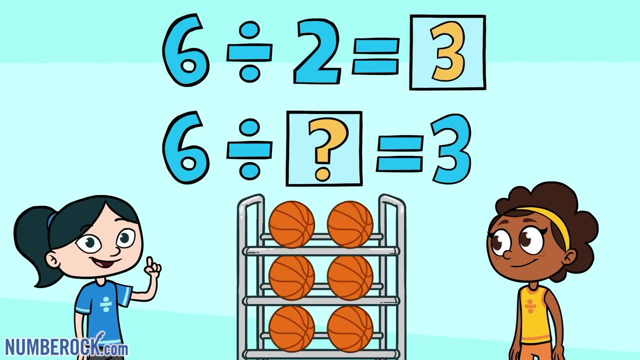 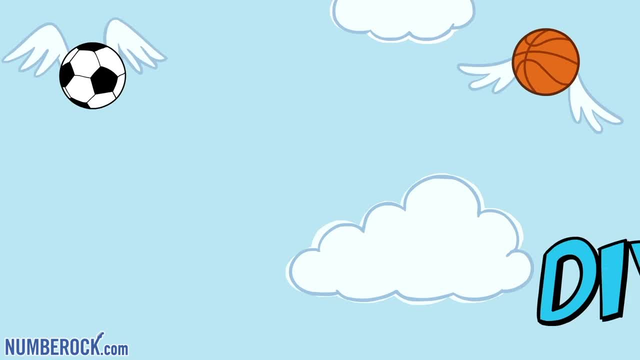 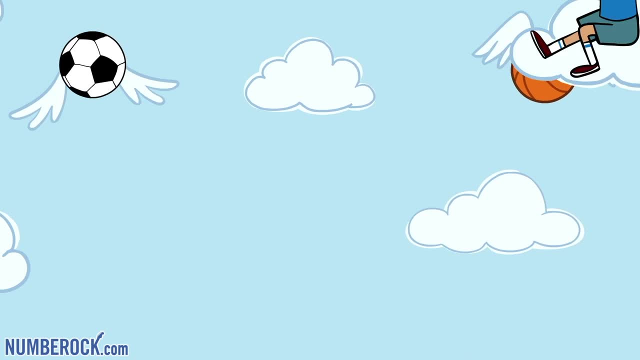 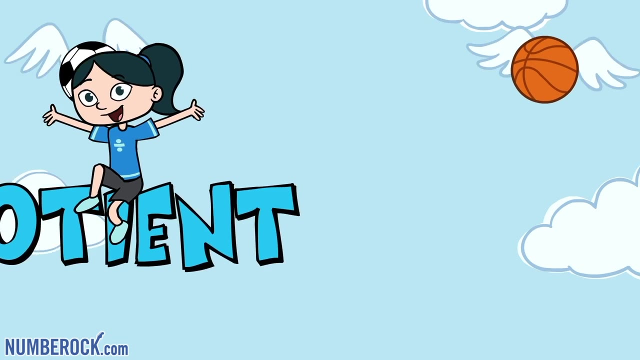 If we look at the basketballs, we can find three groups of two, Or We can find two balls in three groups, Which is equally true. The number divided Is the dividend. The divisor divides, So that in the end We'll find the number of groups. That's the quotient. 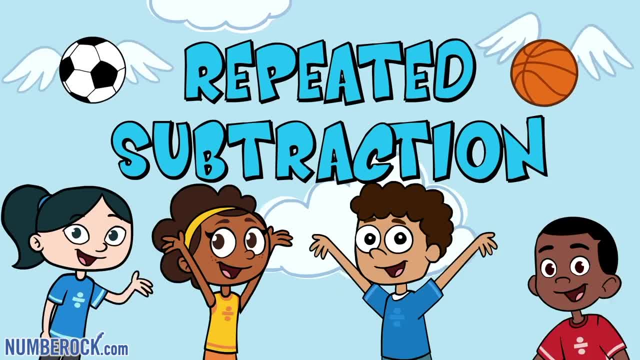 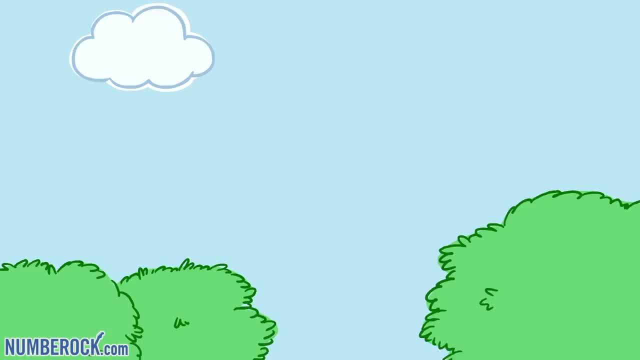 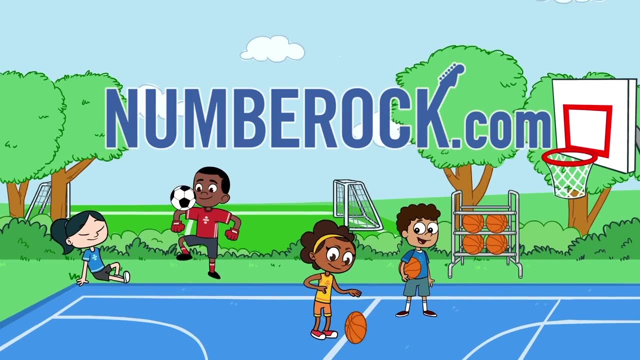 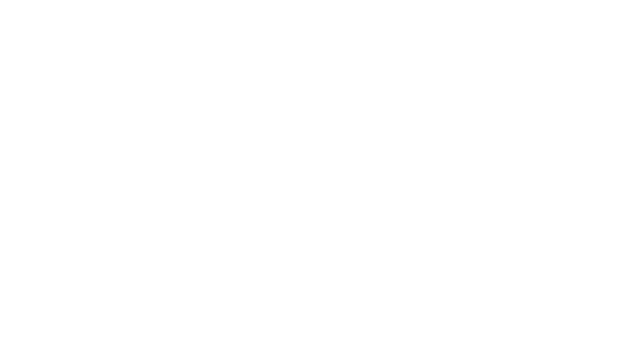 We can think of division As repeated subtraction. We can think of division: Is the divisor divided? In the end, Th jurisdiction. Is the divisor divided? Is the divisor divided? Is the divisor divided In the end, As repeated subtraction. We can count that Hoping Yep One. That's the quotient. How are we going to pass tack? What about the following? Oh unpack, Yes, It's изв quin Number meme In espectrum 800: 70.